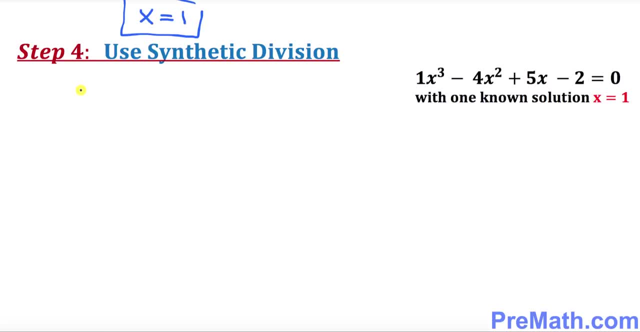 we are going to use synthetic division and the synthetic division- i'm sure everybody knows how to deal with it. so we're going to put down the, the coefficients of our regional equation right up here, which is what one negative four, five, and what negative two, and our one of the solution is: 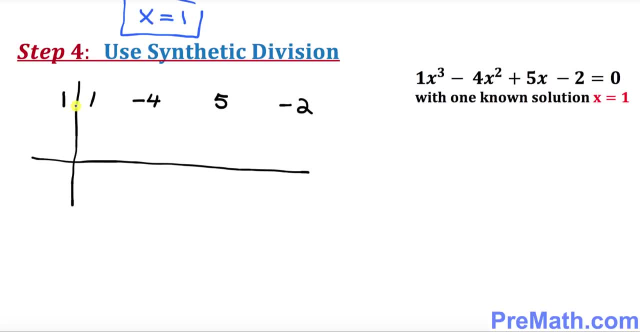 x equal to one. so you must put down one right up here, and let's get started now. so one is you. just put down one as it is right up here. then the next step: i want you to multiply one, this with this one, one time. one is what one i want you. 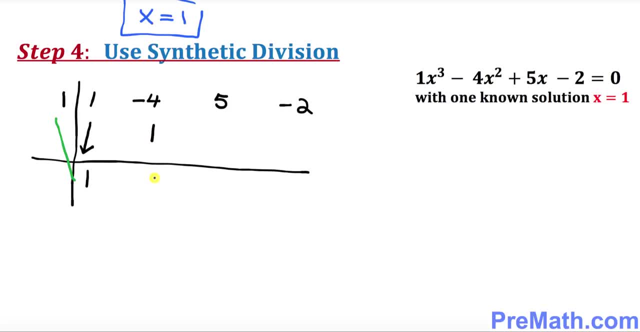 to put it down over here. add negative four plus one. is going to be what? negative three? once again? you multiply this one by negative three. that is negative three times one is negative three. you just put it down over here and add them up. which is going to be how much? two, once again, i. 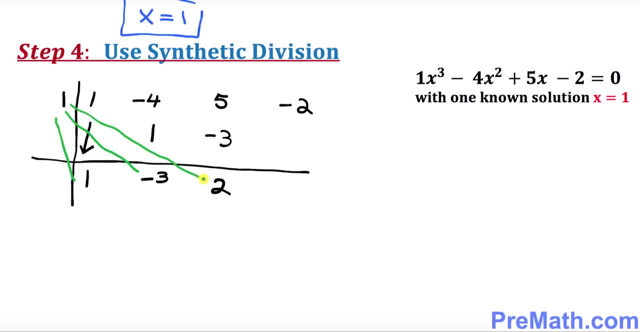 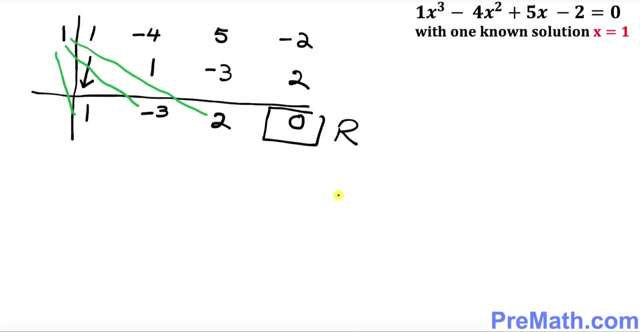 want you to multiply this one times two, which is going to be what? two right up here. negative two plus two is what zero. so zero is our remainder, now what we got next. so the next thing is: now we got these numbers: one negative three and two. so this, the first one, is going to be with the x squared. this is going to be with x and this. 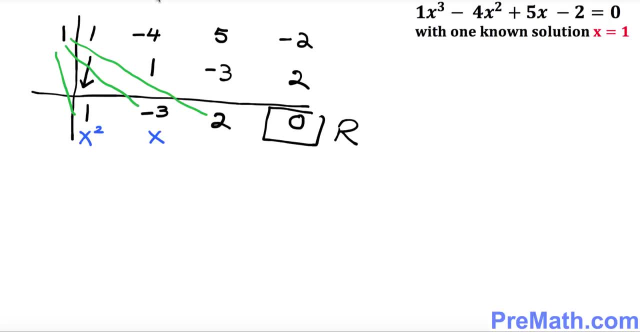 is without x, which is called constant. so, given this one we got, this is going to be what one x squared minus three x, and that's going to be what plus 2, equal to 0, which turns out to be a quadratic equation. so let's go ahead. 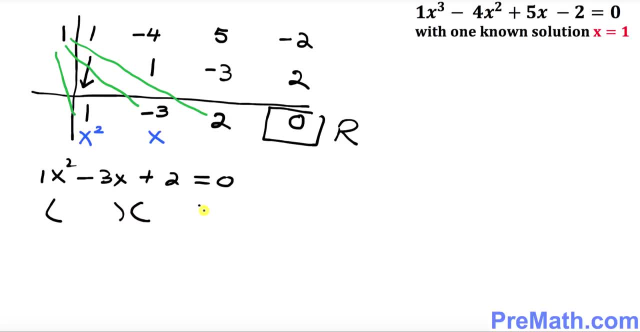 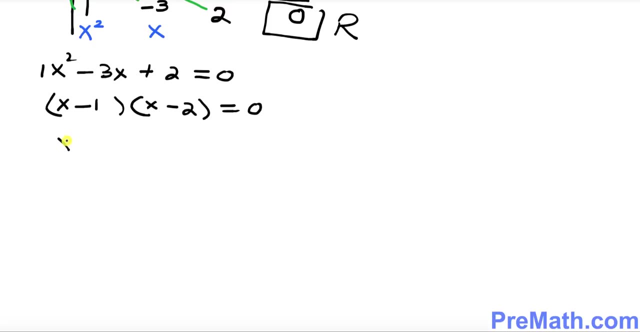 and factor them out and solve for x. so let's factor them out. the possible factors obviously are super easy: x minus 1 and x minus 2. so let's go ahead and split them up right now. so we got x minus 1 equal to 0 and on this side, x minus 2 equal to 0. that tells you that x equals to. 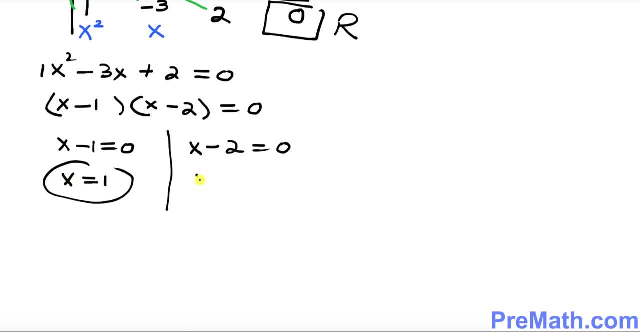 positive 1, and here x equals to what positive 2. so that's what we got, how many solutions we got. so we already figured out one solution in our previous step and we have a two more solution. so that's how many solutions are all together: 1 comma 1 and 2, so they are 3 hour is our solution. 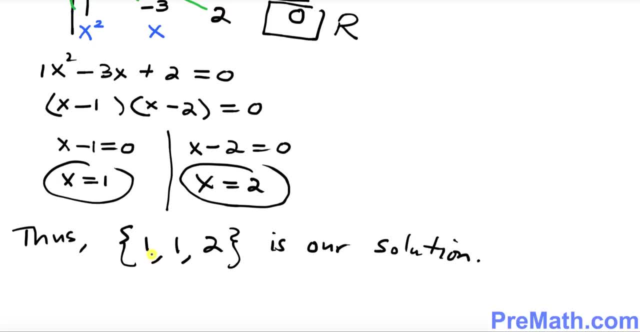 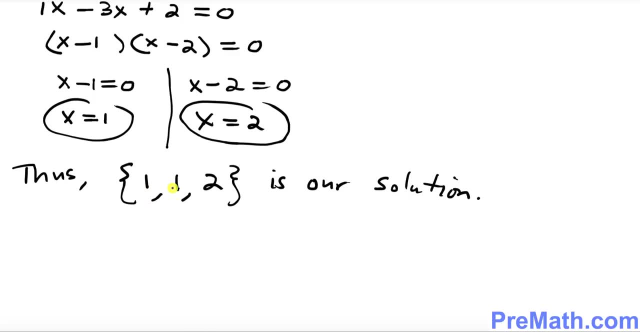 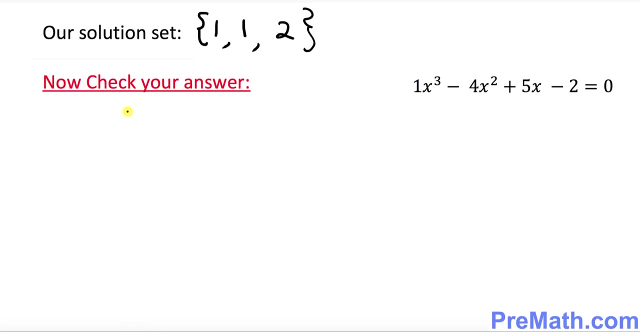 and one thing. I just want to remind you one thing. so the one is repeating twice. so this, this, if one repeats twice, we call it one with a multiplicity of two. okay, just keep in your mind so what we got right now. our solution is this one. and, finally, our final step is to check our answer. so, as you know, our solutions. 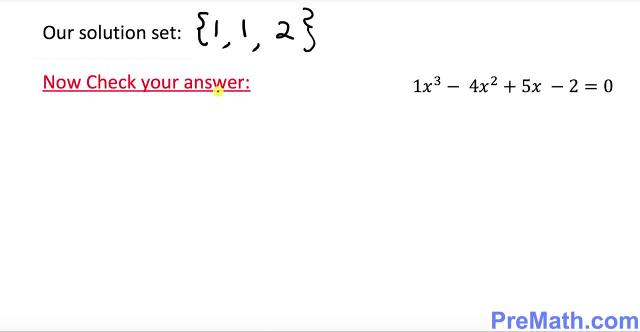 set is what? 1 and 1 and 2.. 1, 1, and 2.. And now, if you want to check your answers, you just simply need to add your solutions up. Okay, so what are our solutions? 1 plus 1 plus 2.. Now it says question mark: is it equal to? 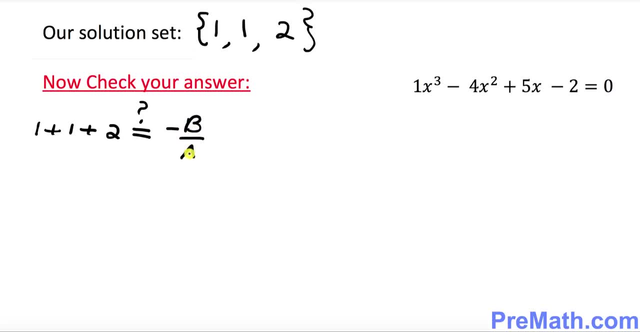 minus b over a, where a is how much. In our case, a is 1,, b is negative 4, c is positive 5, d equals to negative 2. So that would give you negative b over a is going to be simply what? 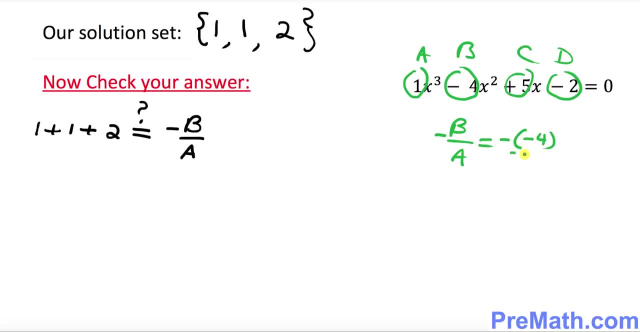 Negative and b is negative: 4 over 1.. So that's going to give you 4 over 1, that is equal to what? 4.. So let's go ahead and check it out. On the left-hand side we got. 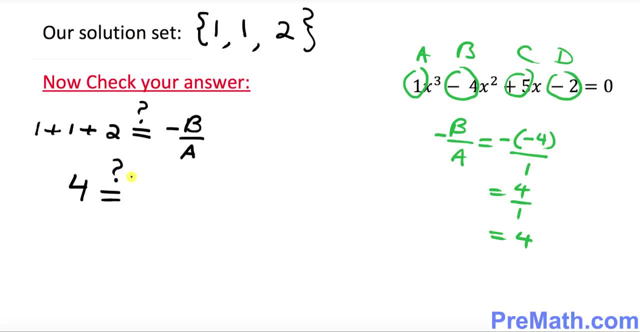 of course, obviously 4 question mark Is the right-hand side turns out to be from. here is what 4 as well Is. 4 on the left-hand side equals to 4 on the right-hand side. That is yes, That means.